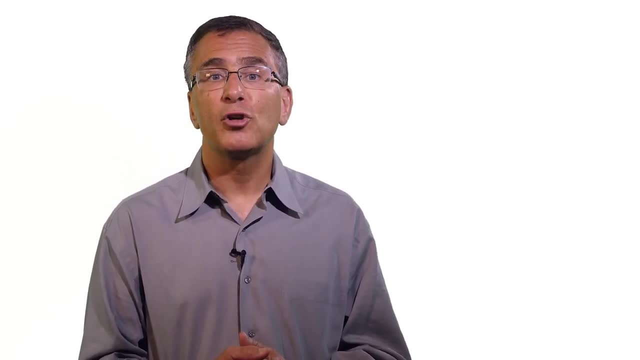 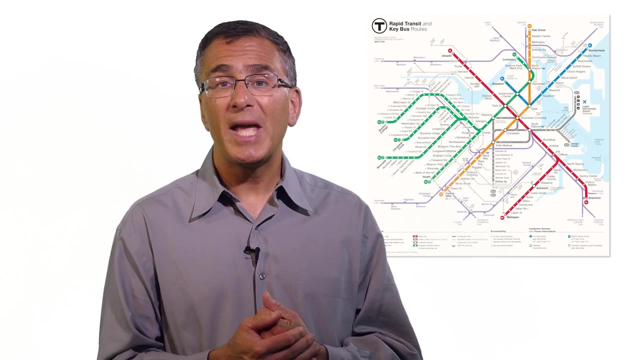 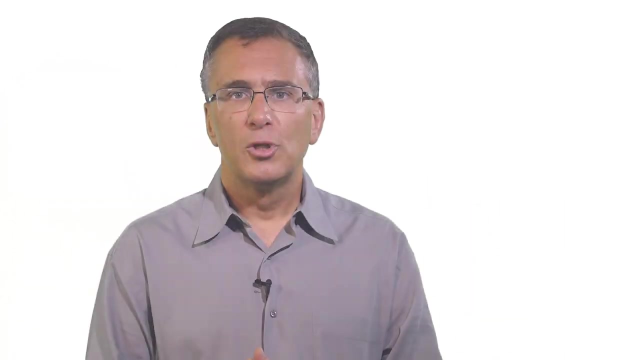 it will be helpful to represent these preferences using a graphical representation. Think about how a subway map condenses a city into lines showing how you get from station to station, Or how an emoji condenses your mood into a single smiling yellow face. We'll use the same strategy to represent your preferences. 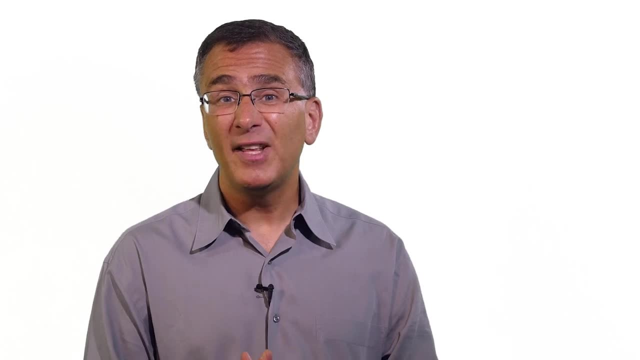 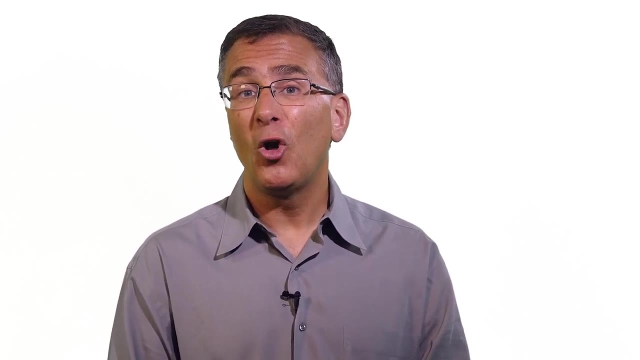 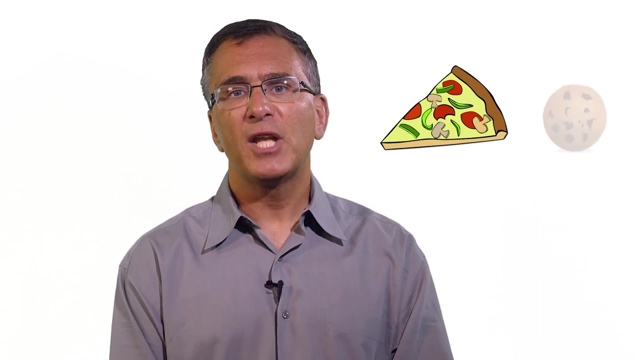 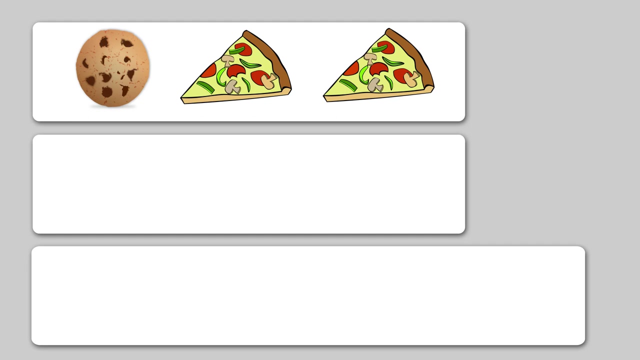 Condensing your feelings about goods into a simplified map that reflects your preferences for one good versus another, A map that we'll call indifference curves. Suppose you're out to dinner and the only items on the menu are pizza slices and cookies. Consider three choices: Two slices and one cookie. one slice and two. 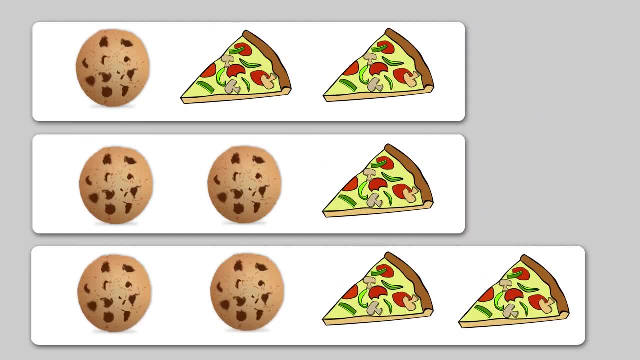 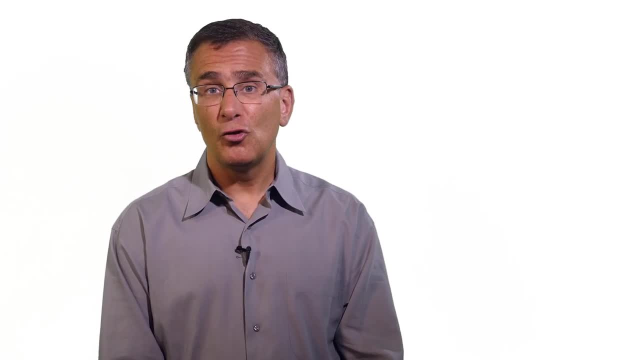 cookies, or two slices and two cookies. Remember, more is better than one. So you prefer the third option to the other two. But let's assume that you're the type of person who is just as happy with either of the first two options, That is, you're. 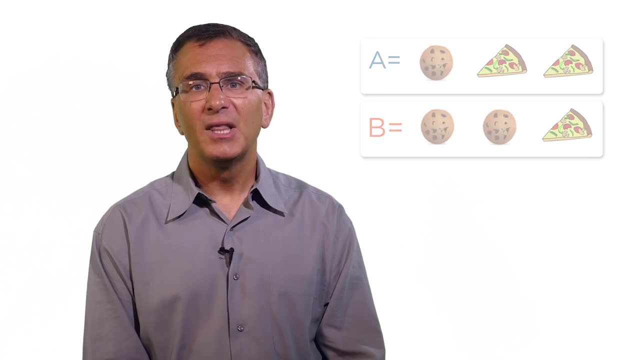 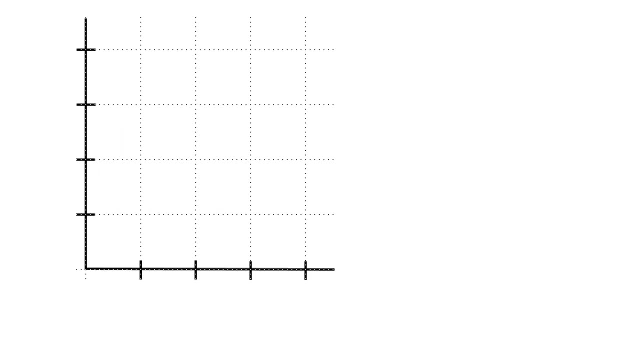 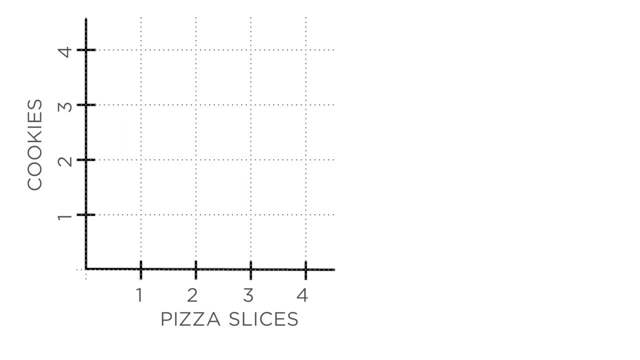 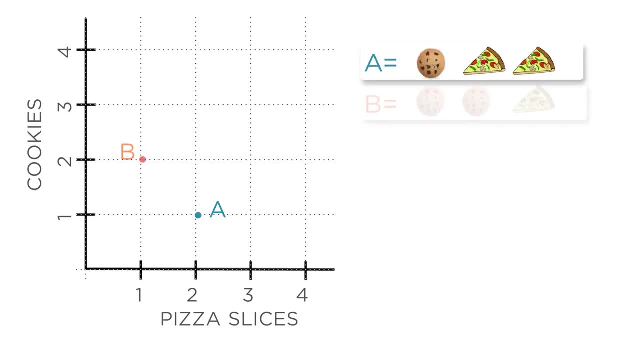 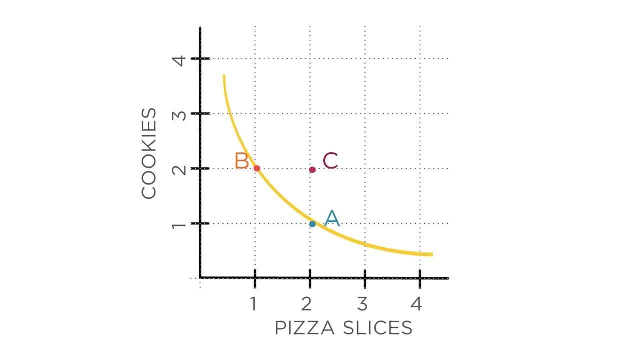 on the y-axis, And B and C go here and here. Next, since you're just as happy with bundle A as you would be with bundle B, we can draw an indifference curve that passes through points A and B. All points on this indifference curve, including A and B, represent bundles. 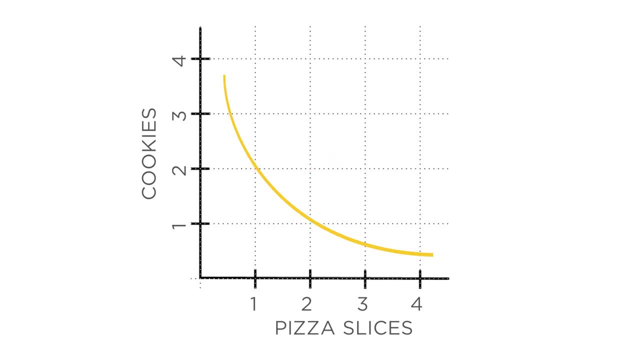 between which you're indifferent. You'd be just as happy with one pizza and two cookies as you would be with half a slice and three cookies, or with four slices and half a cookie. What about that option of two slices and two cookies? Well, you prefer that option to any.